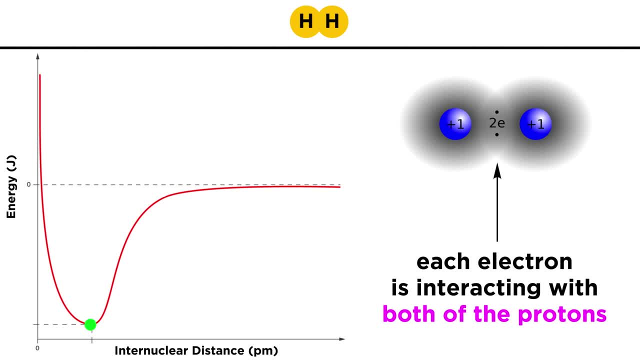 for a molecule of hydrogen. This decrease in potential energy occurs because of the distance between the two protons. This is the ideal distance between the two protons and therefore the precise bond length for a molecule of hydrogen. This decrease in potential energy occurs because each electron is interacting with both protons. 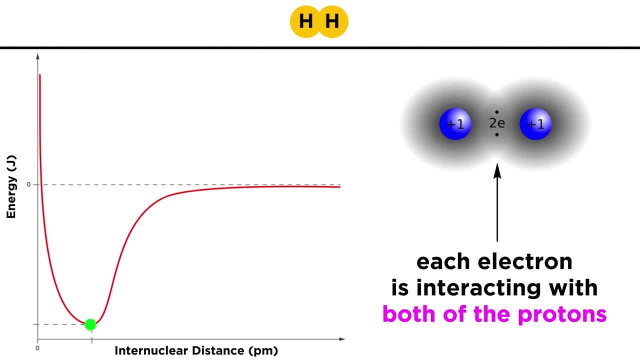 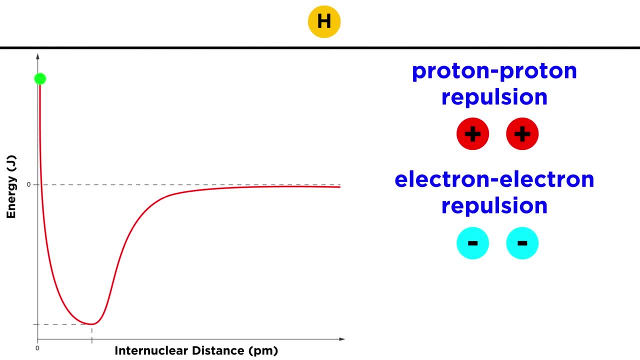 and this is a stabilizing and therefore energetically favorable situation. However, if we continue to push the protons together, things become less favorable due to cumulative proton-proton repulsion and electron-electron repulsion, which will quickly begin to outweigh any proton-electron attraction. 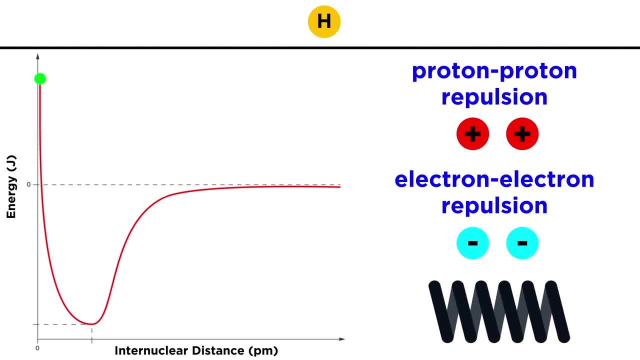 This is sort of like if we were to compress a spring beyond its average current- about a quarter of its current current equilibrium position, and this is why we see the curve rise steeply to the left. So, as we said, it is this phenomenon that reveals the internuclear distance that offers. 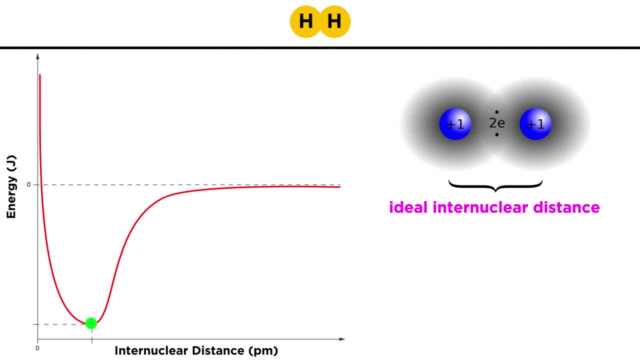 the lowest potential energy and therefore the ideal covalent bond length for the hydrogen atoms, which, for this case, will happen to be 74 picometers, where a picometer is a trillionth of a meter. This also shows why covalent bond formation is always an exothermic process, because there 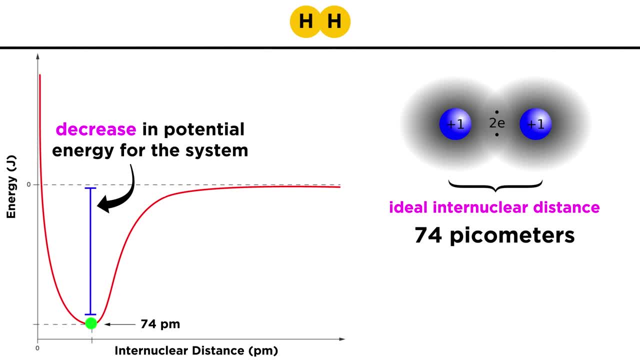 will always be a decrease in potential energy as a result of this kind of orbital overlap, and that difference in energy must be released to the environment. This is also the energy that is required to break the bond, and it will be equal to 7.24. 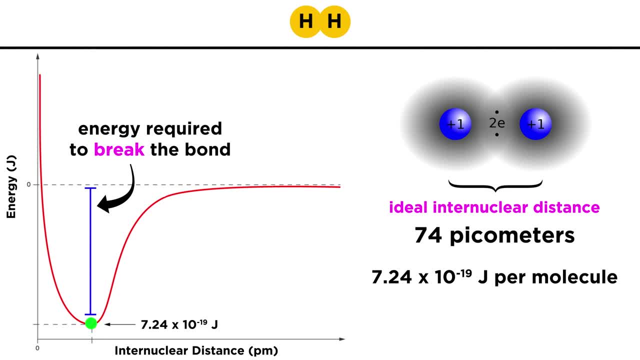 times 10 to the negative 19 joules for one hydrogen molecule. That's a very tiny energy, But multiplying by oxygen, Avogadro's number gives us the energy required to break the covalent bonds in a mole of hydrogen molecules. and that will be 4.36 times 10 to the 5 joules which becomes. 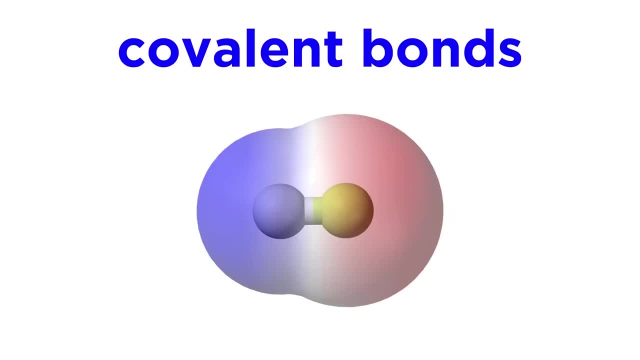 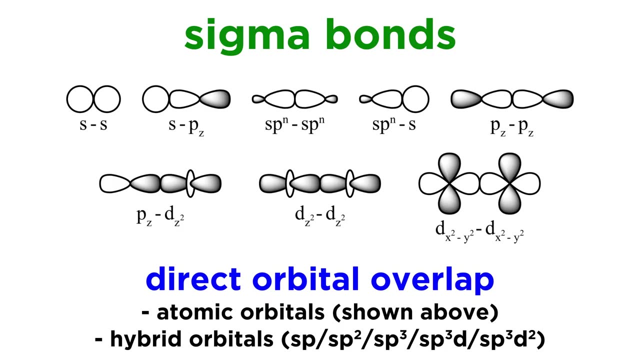 quite significant. In this way, we can look at any covalent bond in a slightly more sophisticated way. Sigma bonds involve direct orbital overlap, and this can be between atomic orbitals or between two hybrid orbitals, be they sp, sp2, sp3, and sp4.